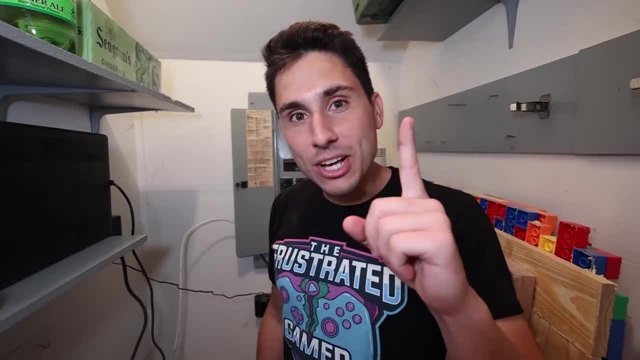 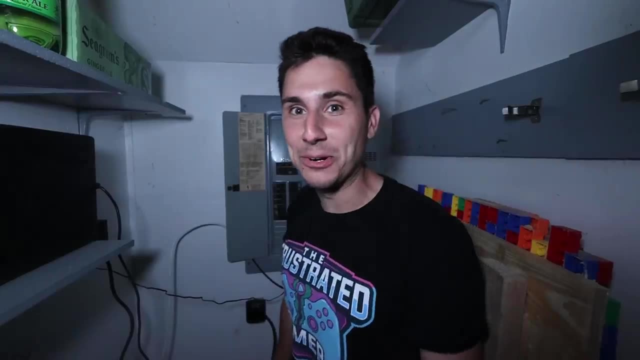 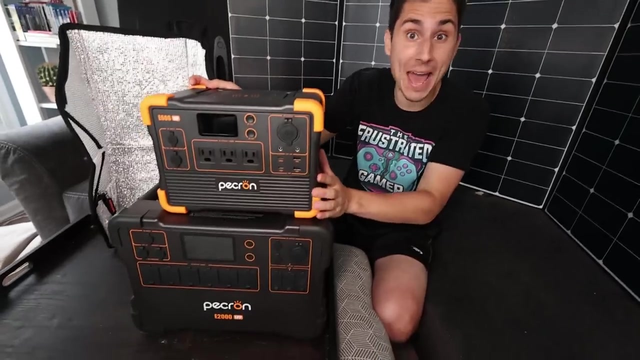 Sam is not happy about this idea at all. Our one week on only solar power begins Now. So these are some of the tools I'm going to be using to survive the next week. I have two big solar panels, I have two Pekron batteries and then this weird contraption. I'll tell you. 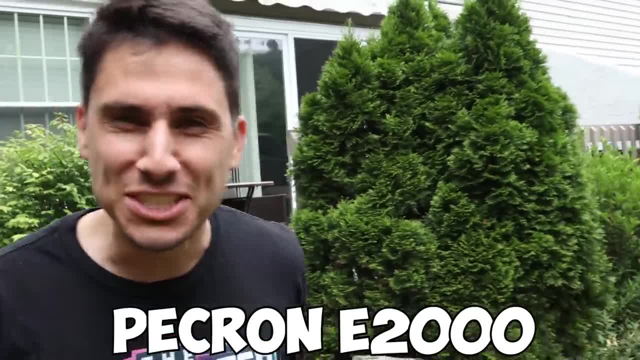 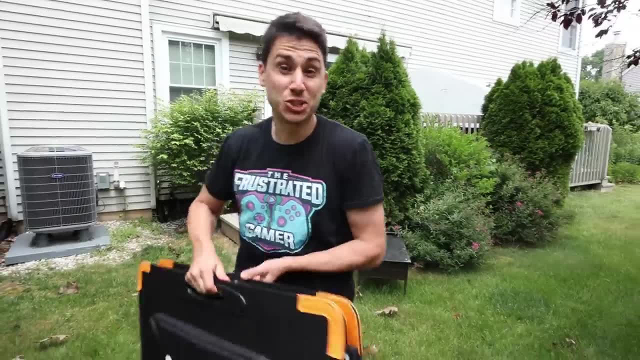 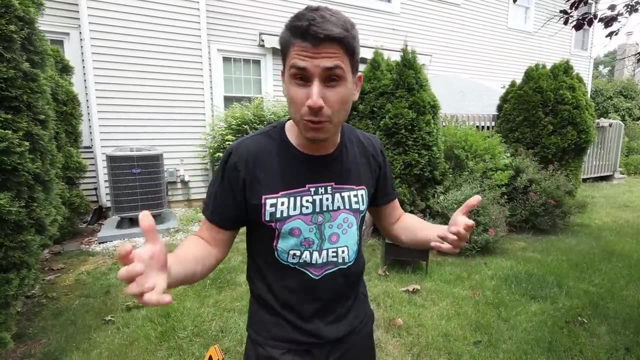 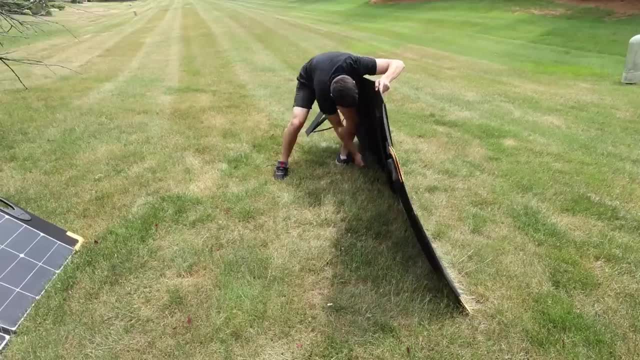 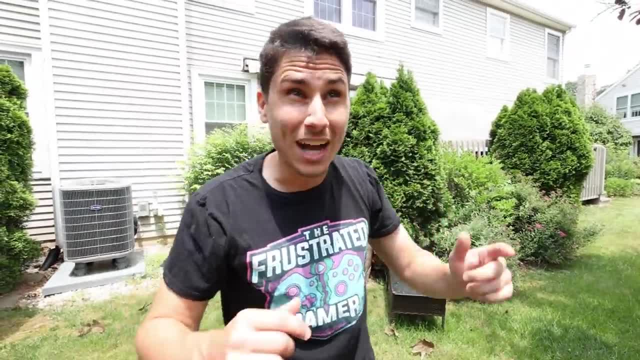 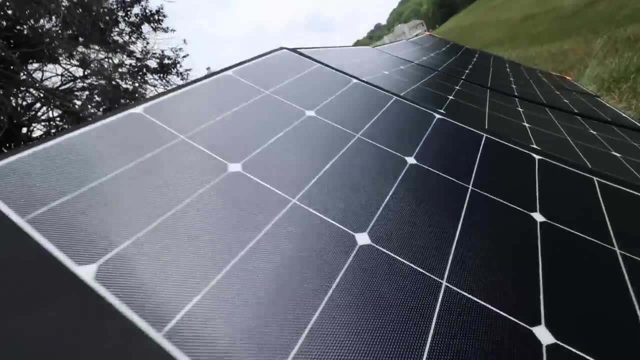 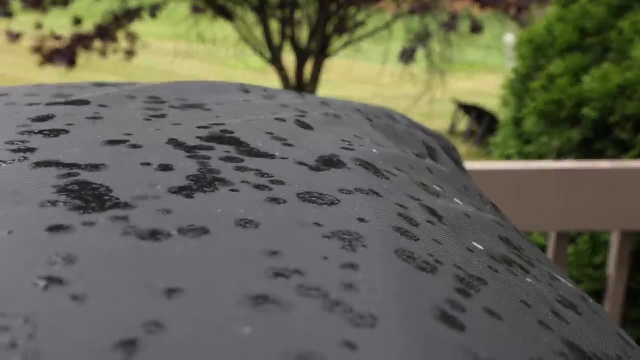 It's working Okay. So right now we're getting 244 Watts. The sun is getting stronger, so that's going to raise. Also, my refrigerator is off right now, so I really need power fast. So the battery has been charging for about three or four hours. 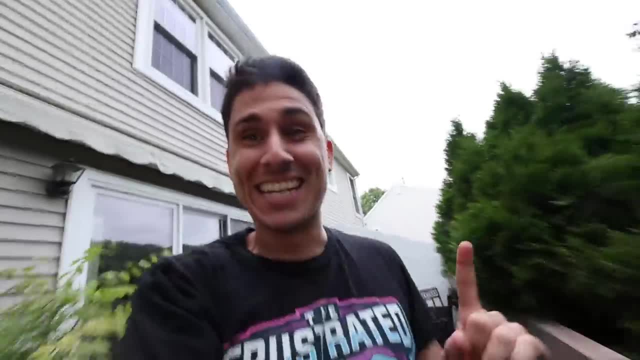 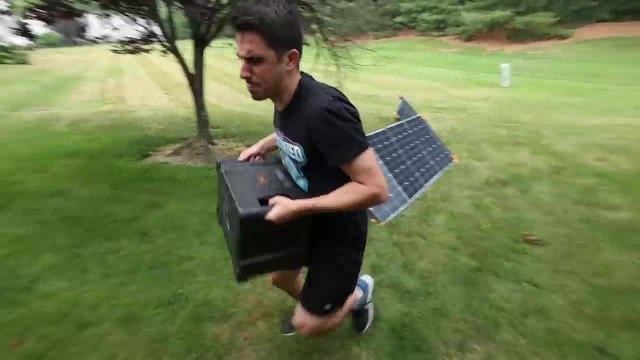 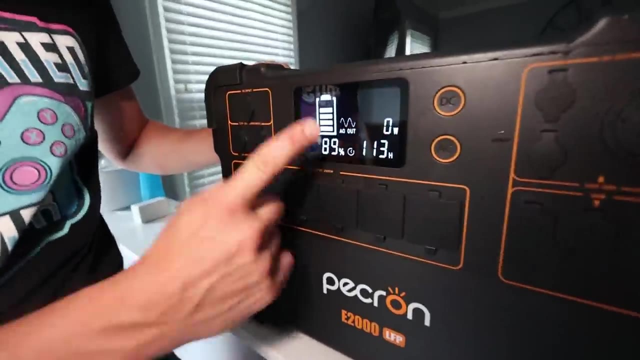 So the battery has been charging for about three or four hours And I looked outside and it just started raining. I don't know how waterproof these things are, but I am not taking a chance on day one. Okay, Let's see how much we charge the big battery. We got it to 89%. Okay, That's actually. 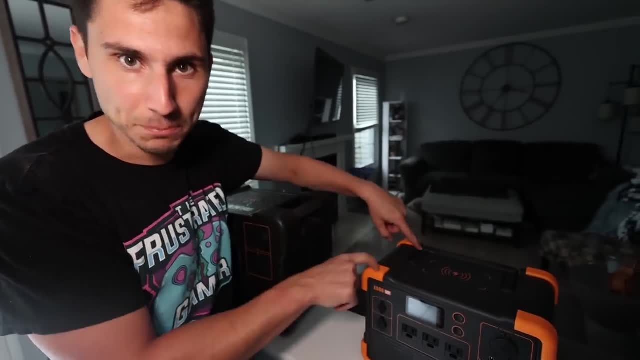 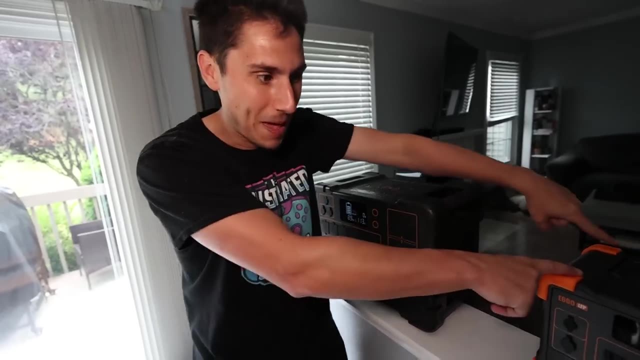 pretty good. The bad news is I didn't get a chance to charge the little Pekron. My plan was to use this Pekron to keep the refrigerator running. I'm going to try to charge the little Pekron with the big Pekron, just enough so I can power the refrigerator. I've got a lot of ice. 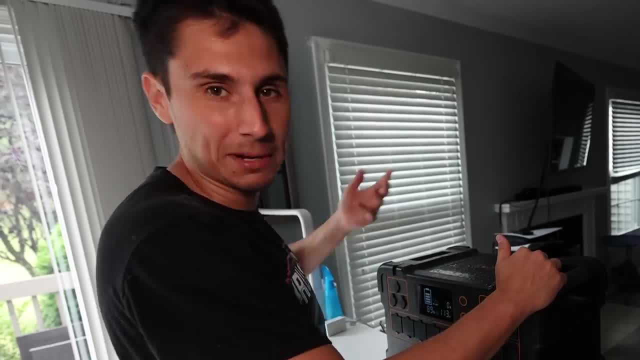 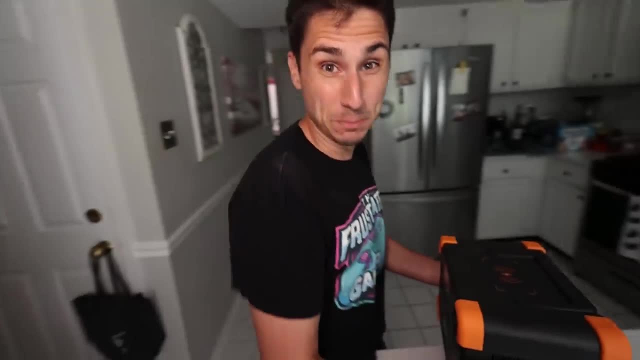 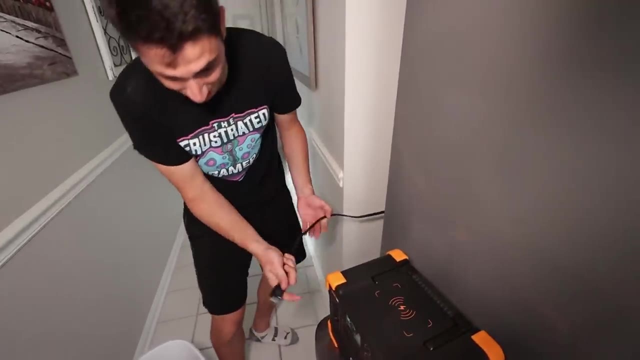 cream in my freezer. I don't want it to melt. Also a lot of milk and eggs and other things that aren't as important as ice cream. So this has been charging for a little bit over an hour. 66%, That's actually really good. I think I heard it. come on All right. 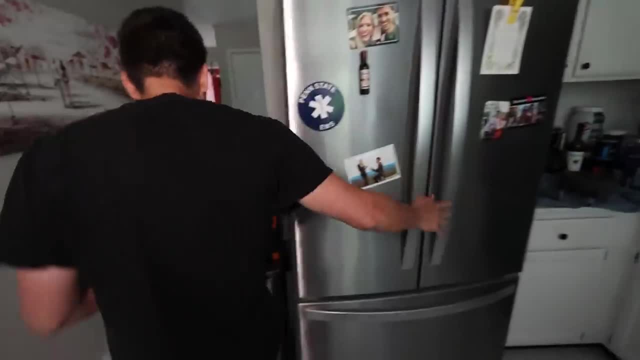 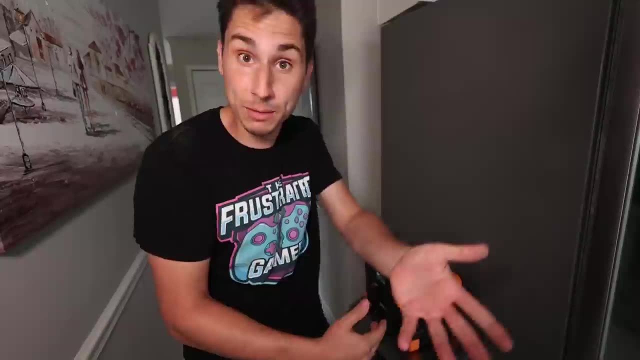 Oh yeah, Power Dude, this is so cool. So this one is the Pekron E600.. It's a little bit smaller, It's a little bit more affordable and it still works really well. So I'm going to keep the. 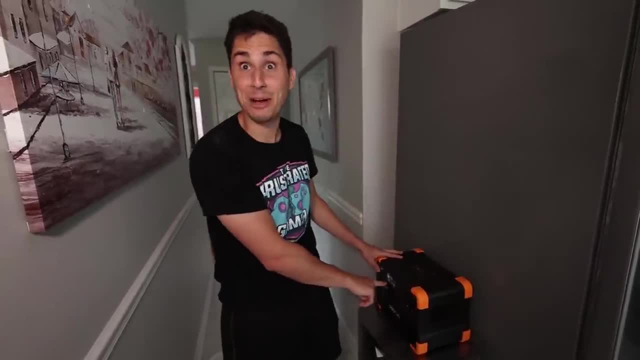 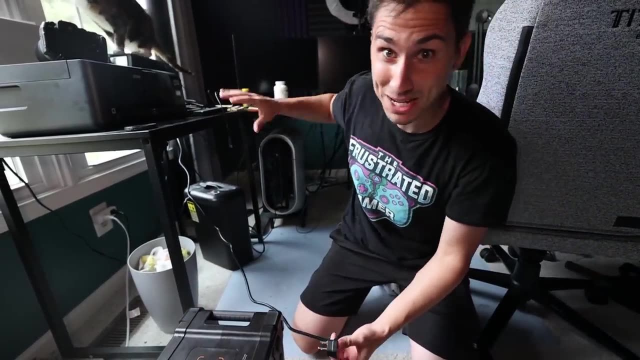 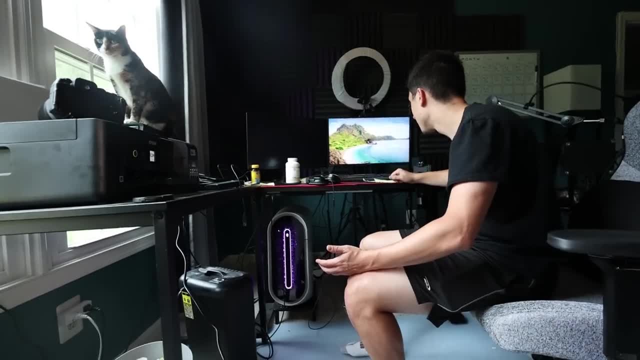 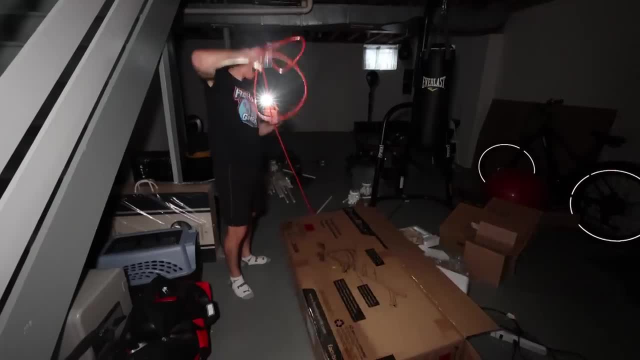 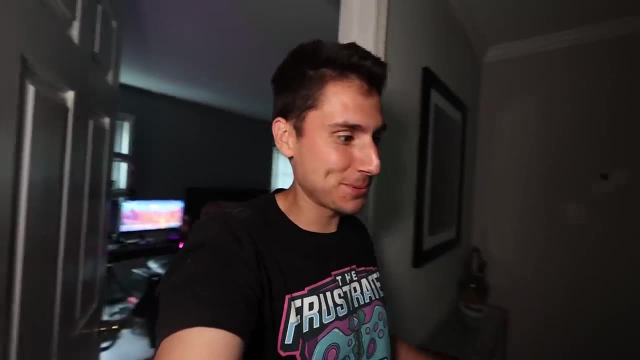 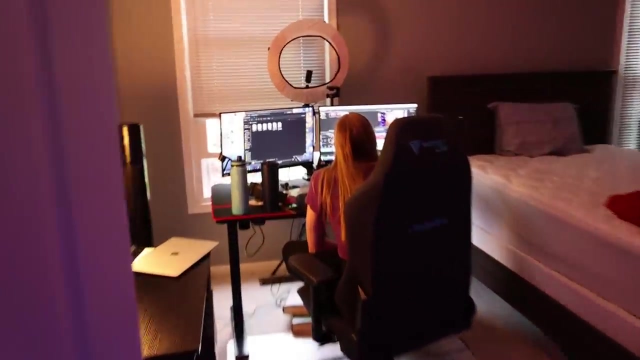 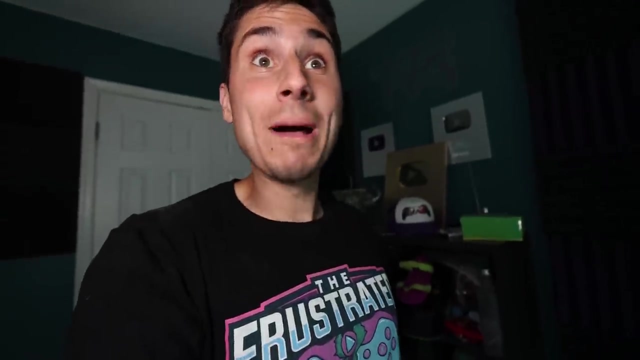 Oh yeah Yeah, We got to plug yours in too. We are fully powered up, all with solar power. I think that's pretty cool. One thing we do not have is air conditioning. not going to have that. for the entire week. It's very warm outside. That's going to be the only. 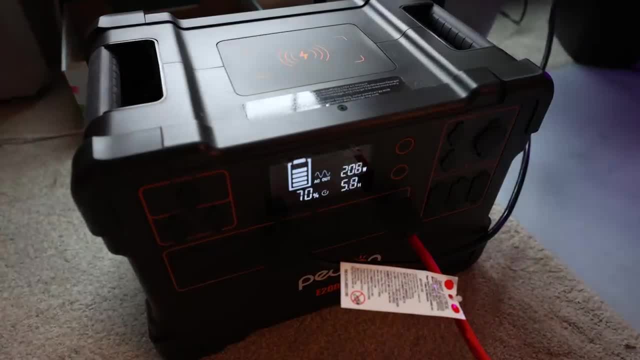 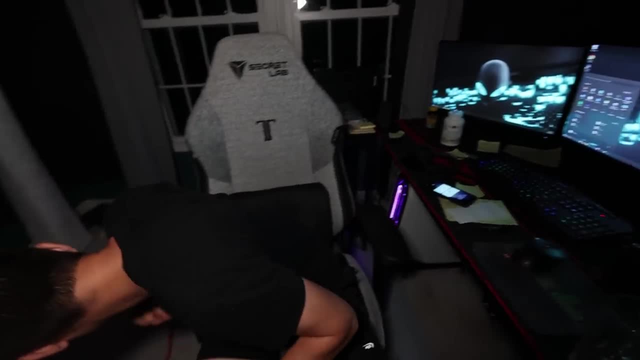 problem. Okay, so it's about 9.30 at night on day one. I'm going to shut my computer down. We have 36% left on the big Pecron- The small Pecron's still downstairs powering the refrigerator. 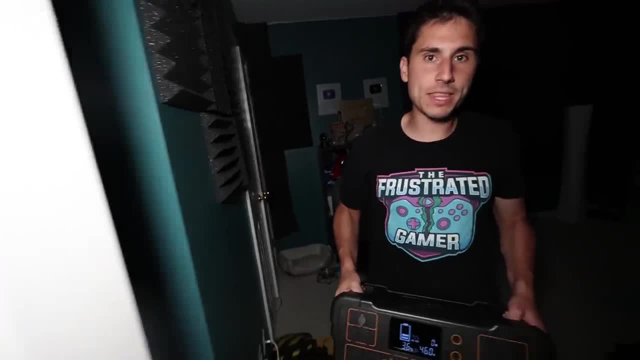 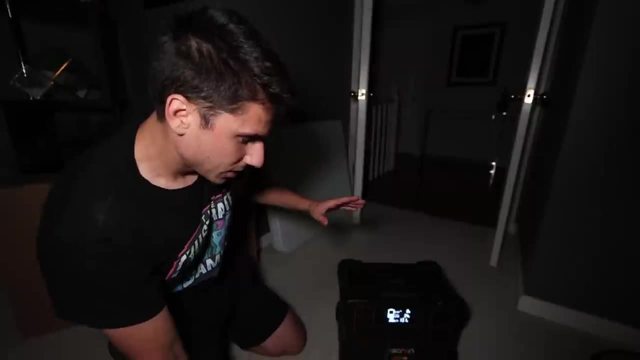 It's like 80 degrees in my house right now, so I'm going to bring the Pecron to my bedroom. I have a fan, but I don't know how much power the fan uses- 34 watts, Okay, that's good. It says we have 13 hours of fan usage. I also want to charge my phone. 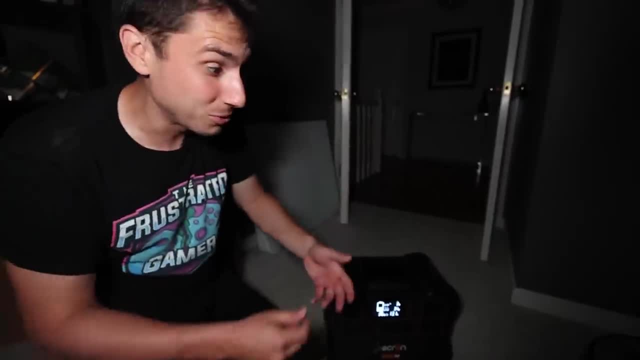 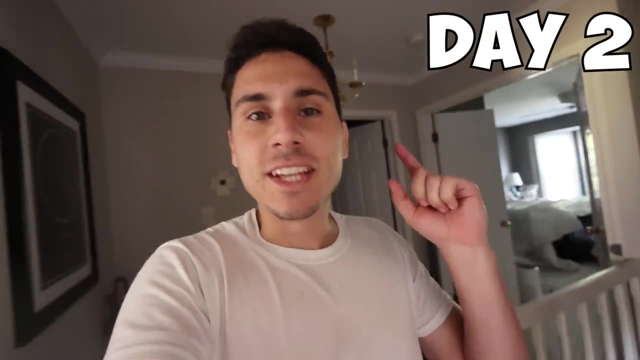 It's got a wireless phone charger right on top. I should wake up tomorrow with the fan on a fully charged phone and hopefully the sun will be up and we can charge this thing up again. So it's the morning on day two. My phone is fully charged, but the Pecron is basically. 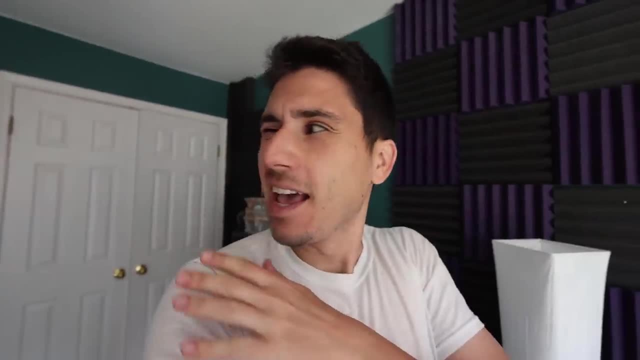 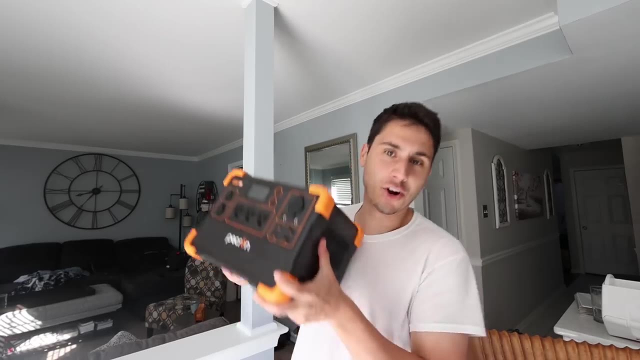 completely out of battery. I also checked the Pecron downstairs and that only has about 8% left. The good news is the sun is very bright today, So I'm actually going to start by charging the little guy, just so I can get the refrigerator back up and running. 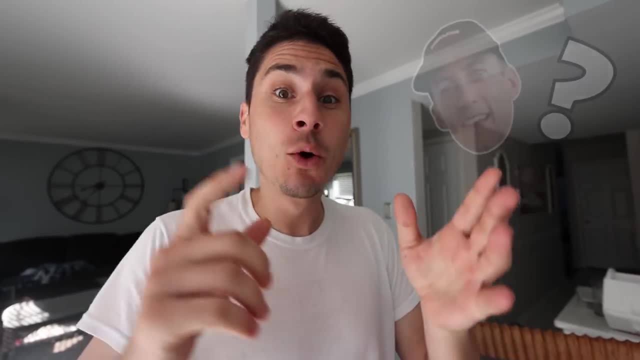 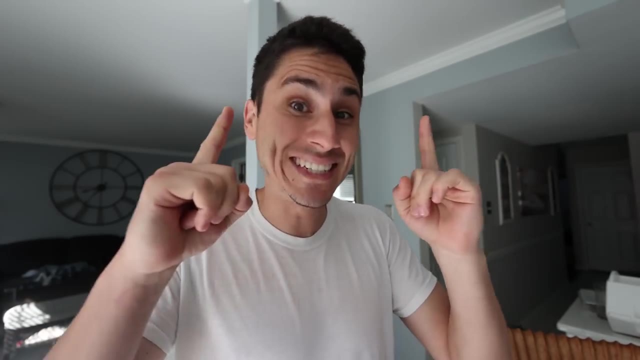 But really quickly I wanted to mention you might be wondering where is Steve? Well, Steve just got married a couple weeks ago. He's currently in Europe on his honeymoon, but he's going to be back by the end of this video And what he doesn't know. I'm going to be surprising him with this. 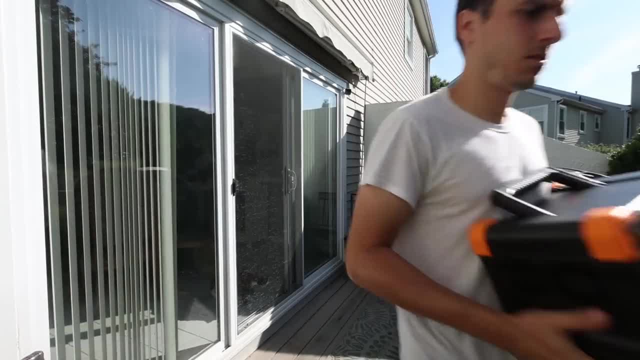 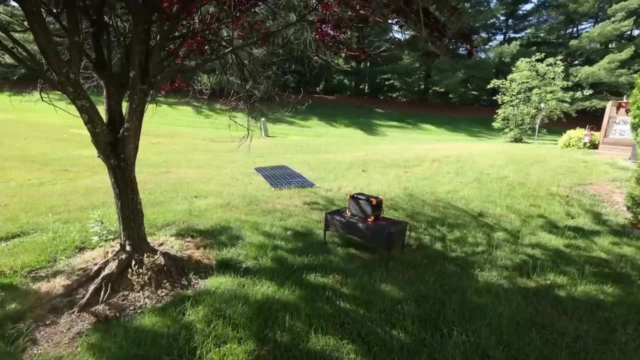 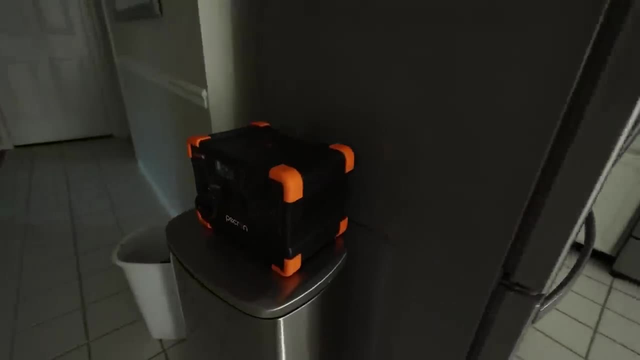 brand new Pecron. It took about five hours but I was able to fully charge both of the batteries with the solar panels, Just like yesterday. I hooked up the smaller battery to the refrigerator and the bigger battery I put up here in my office. Luckily, Sam was at work all day so I didn't. even have to share my power with her, So the big battery was more than enough to last me the entire day. Day three was a rough day. I was able to charge the small battery for about 45 minutes in the morning and then pretty much the rest of the day it rained. 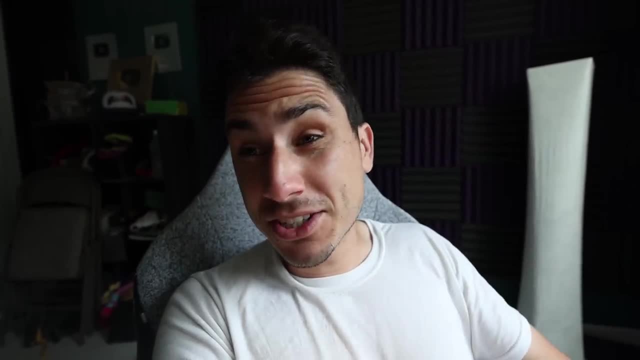 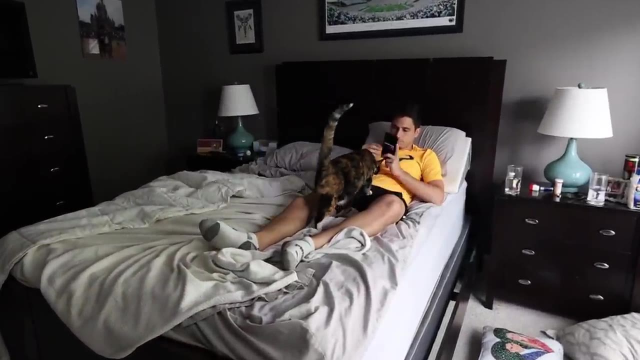 I had about three hours of battery left on the big battery, so I got a little bit of work done. I worked on one YouTube video and the rest of the day I kind of sat on my phone and hung out with Roxy. The only nice thing about all this rain is it's finally cooled everything down. 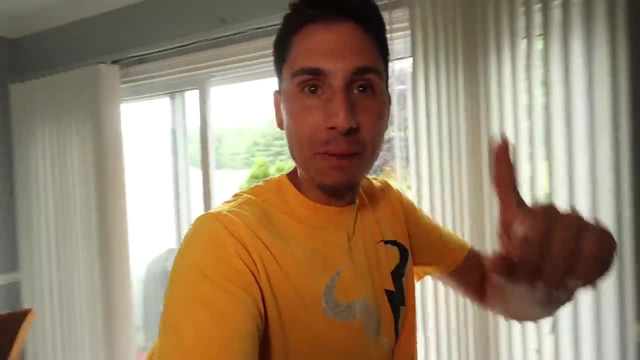 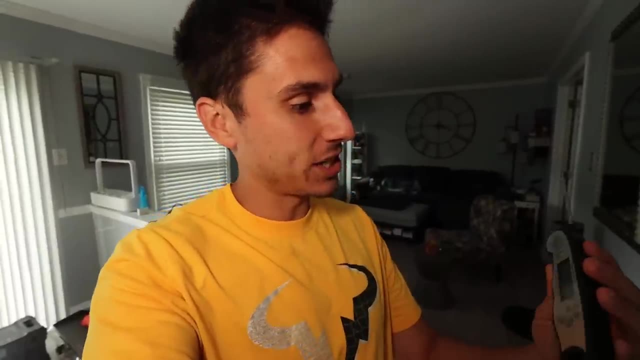 and our house is no longer 80 degrees. I got a little thermometer Let's see how hot the house is. Yesterday the house was up to 80 degrees. It was like 79.8 degrees. What is it right now? 71.6.. That is very comfortable compared to what it's been. 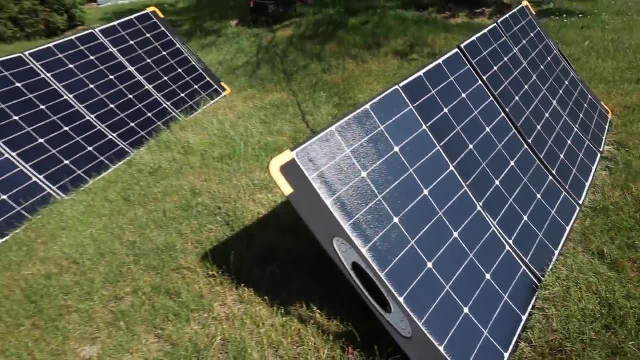 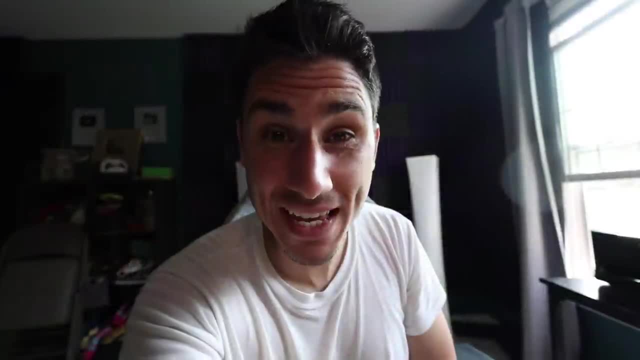 All right, It's day four. Luckily it is a beautiful day outside. Because of all the rain yesterday, I could barely charge either of the batteries, So the big battery is outside charging right now. Today it's supposed to get up to 88 degrees Fahrenheit. 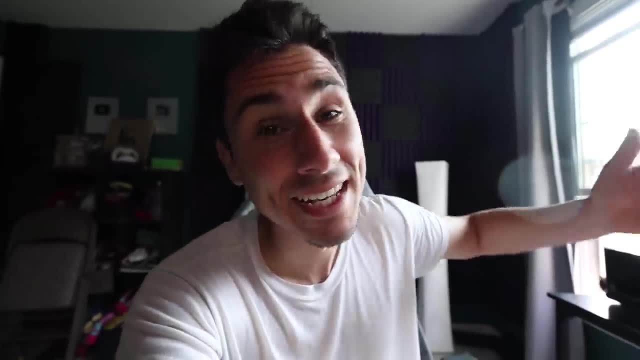 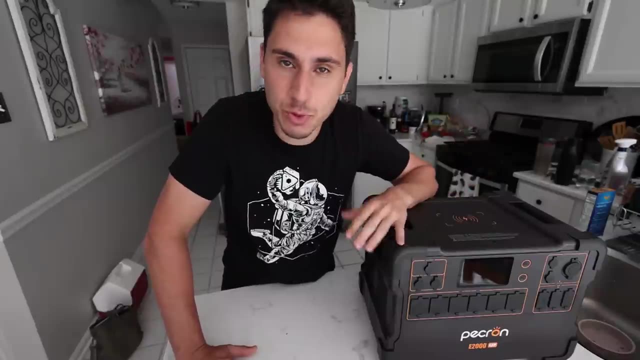 We don't have air conditioning. I have all the windows open, but it's going to get really, really hot in here today, So this thing is almost fully charged. One thing I remembered I haven't been doing for food. Now, honestly, so far I've pretty much just been eating peanut butter and 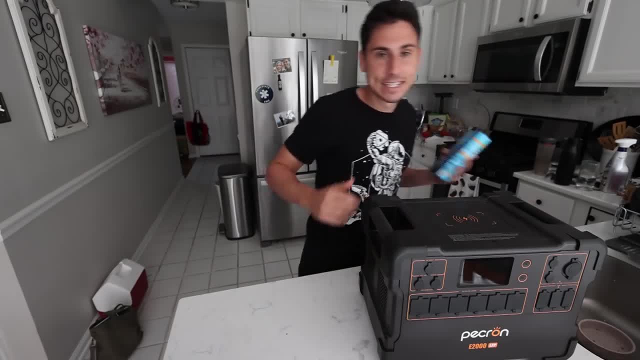 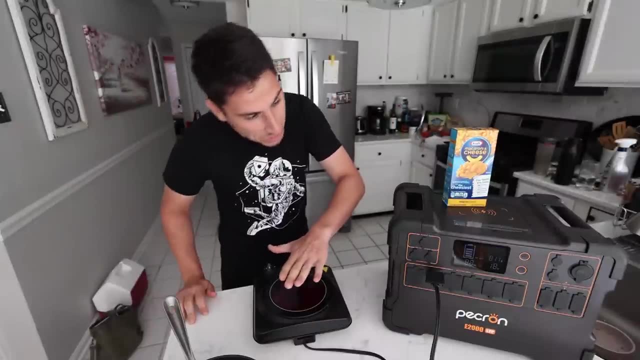 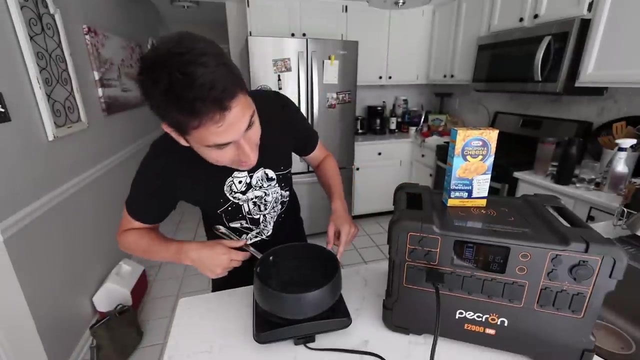 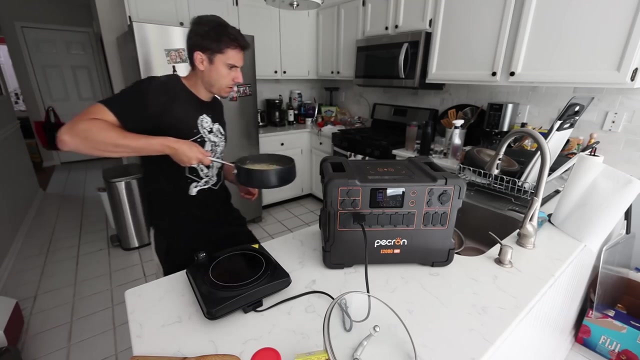 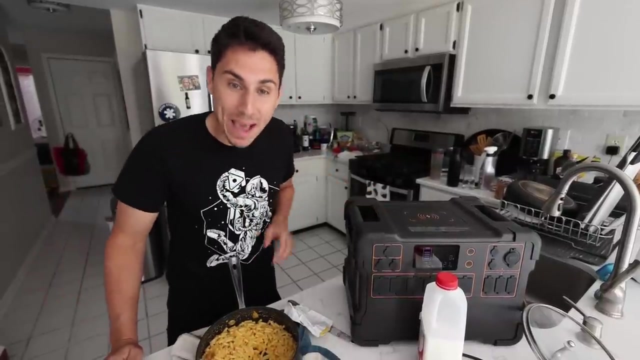 jelly sandwiches, But today I'm actually going to make some mac and cheese. Okay, It's actually working and it is using 810 watts. Oh my gosh. All right, I got to boil this water really quickly, All right. Well, we used like 20% of our battery, but here's the taste test. 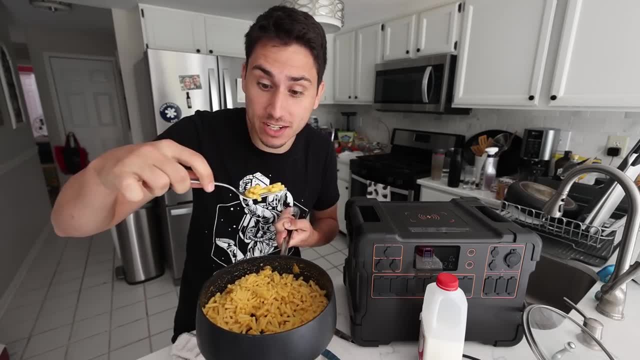 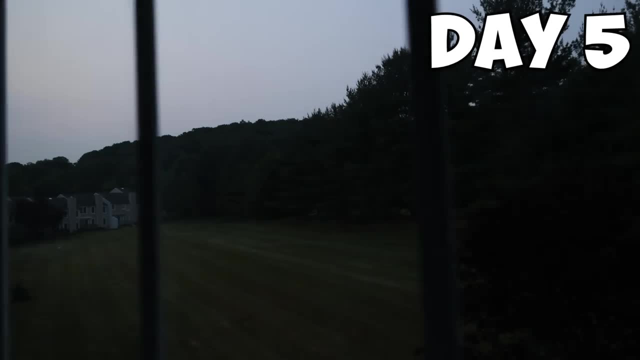 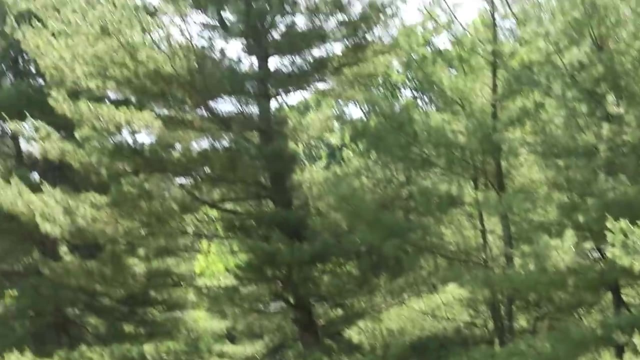 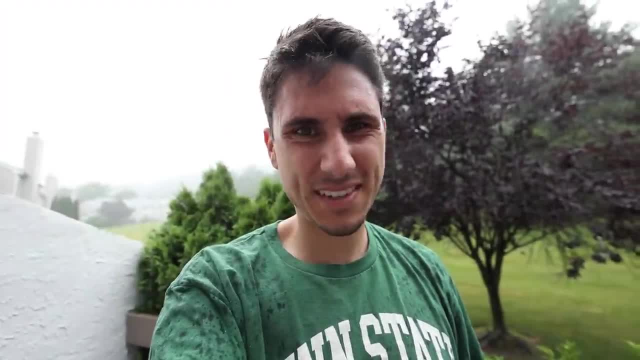 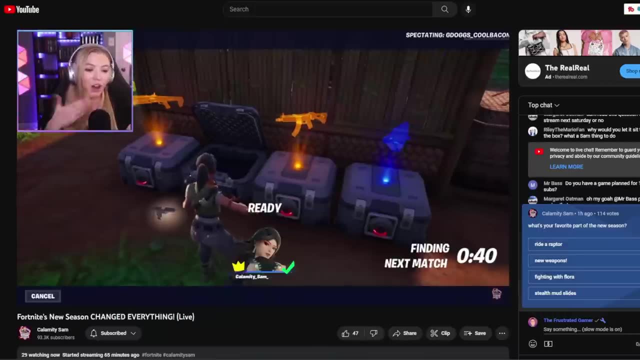 my gosh, Oh my gosh, Oh my gosh. Then it rained for like four or five hours and by the end of the day it was so hot in our house. even Sam was suffering through her livestream. Oh my gosh, It is like 5,000 degrees in my room. 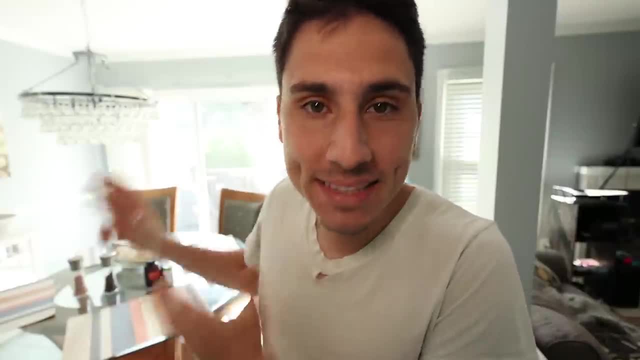 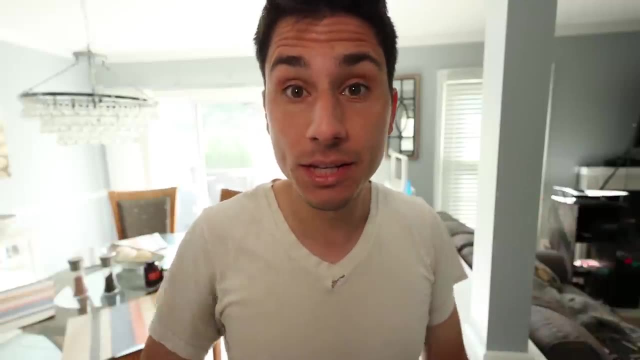 It's day six. The reason why I'm setting up my solar panel on my deck is because one of my neighbors complained that I was setting up solar panels in my backyard. I'm not really sure why. Clearly she is allergic to fun. 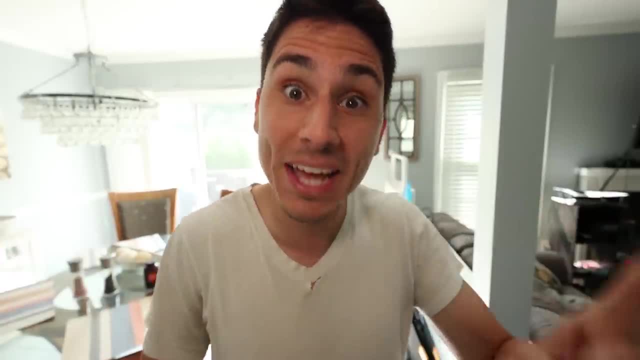 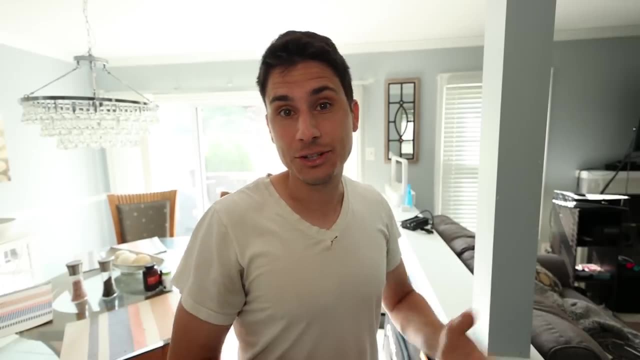 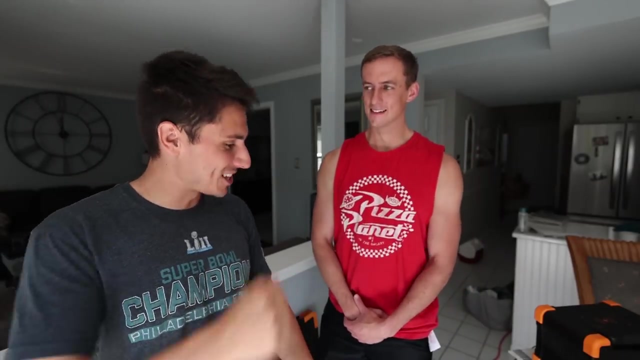 But it's not a big deal. We only have 24 hours left in the challenge, but Steve has come home from Europe. He's actually gonna be visiting my house now. Actually, it's gonna be in a couple hours. Welcome back home, Thank you. How was the honeymoon? 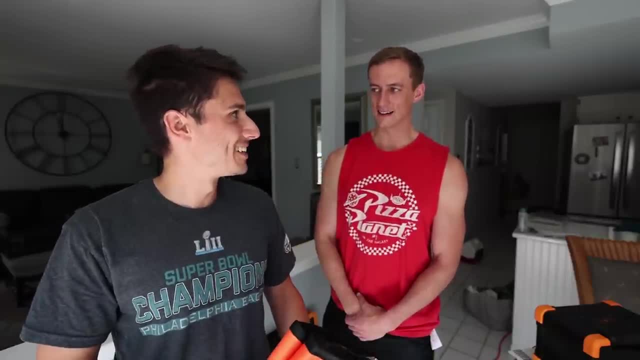 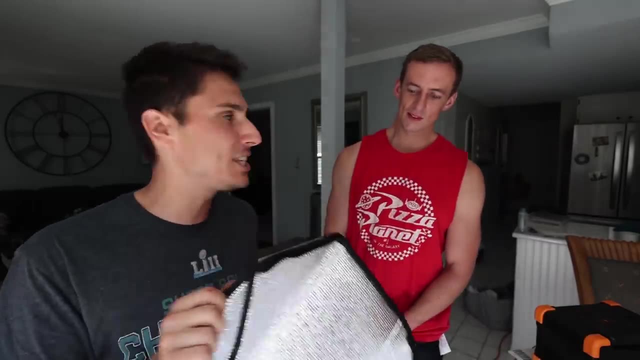 Wonderful. You went to work, Croatia. Yeah, you got food poisoning? Sure did. Yeah, we talked before I turned the camera on. Anyway, enough about that. I hinted that we're using this fun contraption in this video. This is a solar cooker, So it uses no electricity, No solar panels. 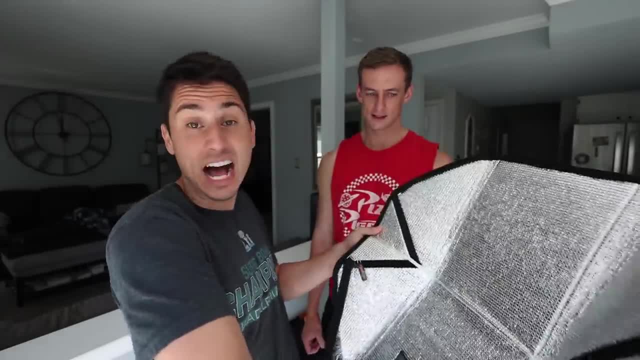 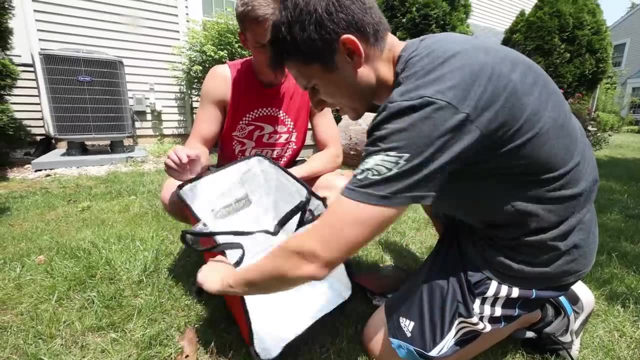 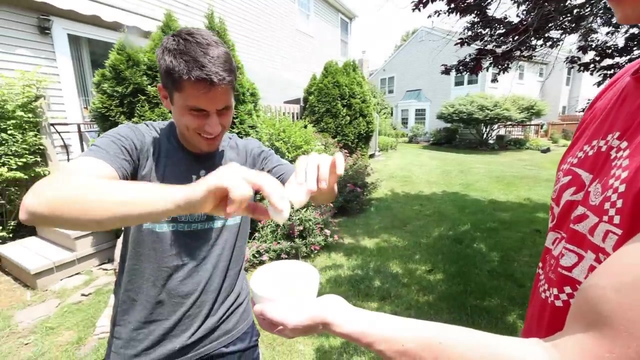 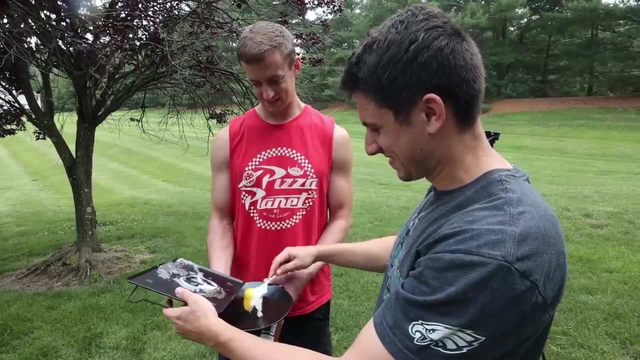 Apparently, if you angle it the right way, you can get it hot enough to cook things. sunny-side up eggs: That's what I want for lunch today. Oh, It's getting warm, is it? yeah, Wow, We cooked a sunny-side up egg, just with the Sun, so exactly seven days ago from right now. 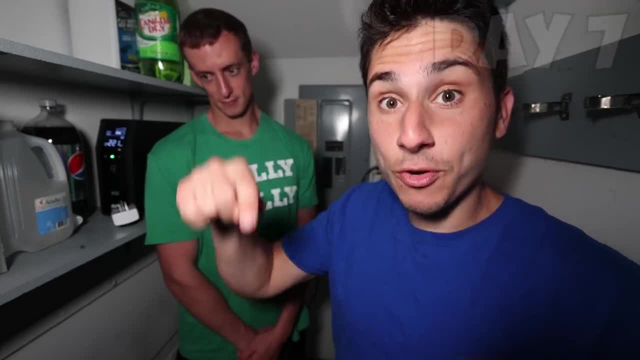 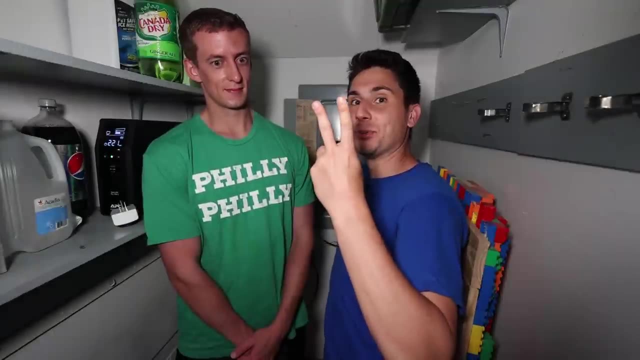 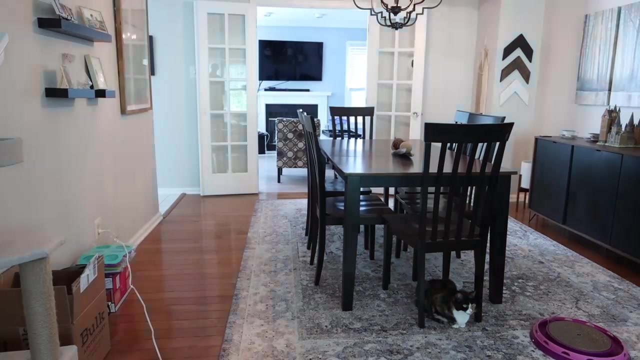 I shut off that switch and we've basically completely lived off of solar power. three, two, one. Oh, it's really hard, But I have a surprise for you. Let's go inside. Pecron was nice enough to send me this box for free, But I have a surprise for you.